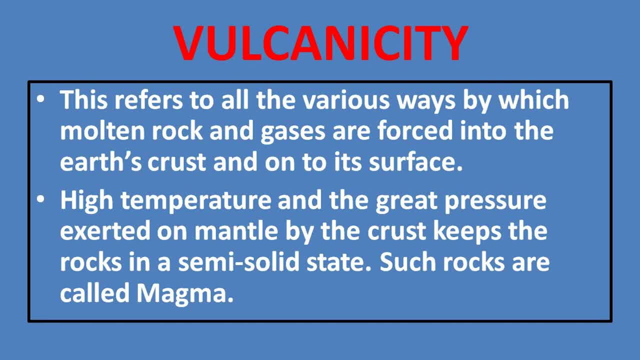 boundaries of tectonic plates raises the temperature, and this, plus a reduction in pressure caused by faulting and folding associated with the movement of tectonic plates, Causes the rocks to become molten and semi-fluid. Such rocks are called magma, so we need to understand how does magma come about to the high temperature and 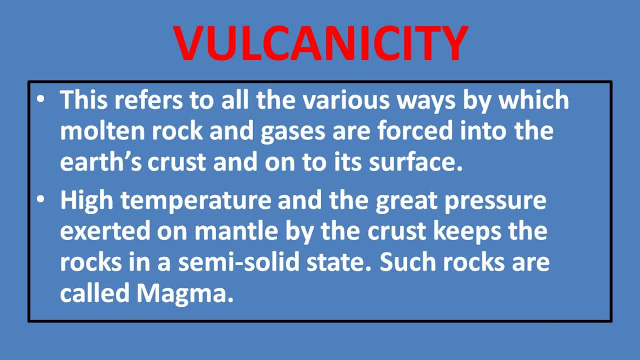 the great pressure exerted on to the mantle. So we are saying, as the magma rises, it forces its way Onto the cracks of the crust which are caused by folding. Remember, And folding The magma may stay in the crust where it forms the batholith, the sills, the dikes, the larch leaf. 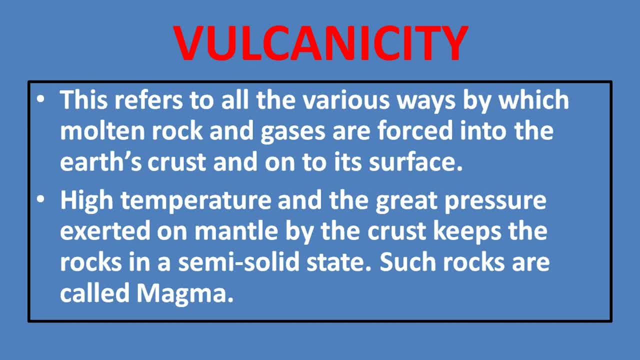 And these are the intrusive It solidifies within. It may reach the surface either quietly or with great violence, as we shall see. If the magma contains a lot of gases, especially the steam, then as the magma approaches the surface, the pressure on the gas is reduced. 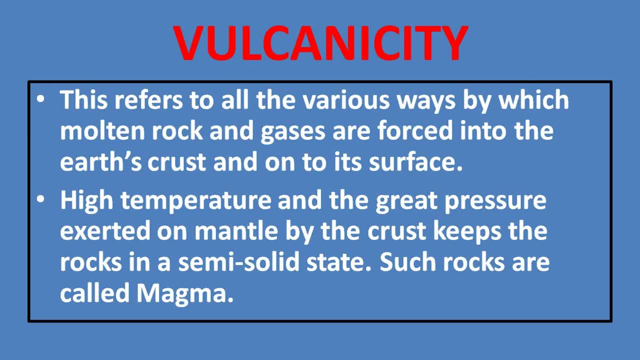 This causes the gases to expand rapidly, which gives rise to violent eruption. So we are saying we have violent and then non-violent. We are going to see that very soon in Alice. So we are saying it is either outside the crust or inside the crust. 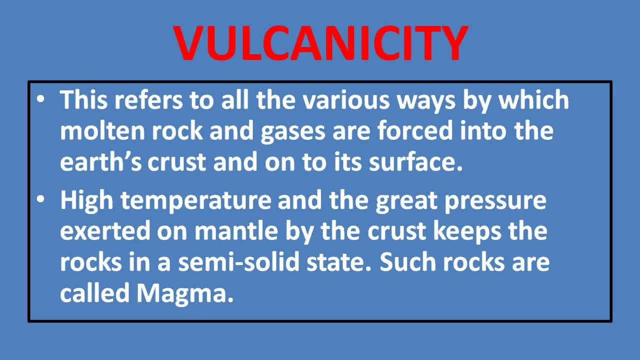 So we are saying the pressure that is exerted on this causes the violent eruption. So when magma reaches the surface, it loses its gases and it is called lava. So what we see on the surface, forming these igneous rocks now, is called lava. 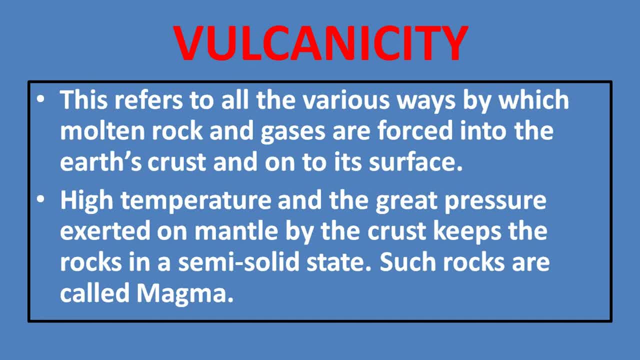 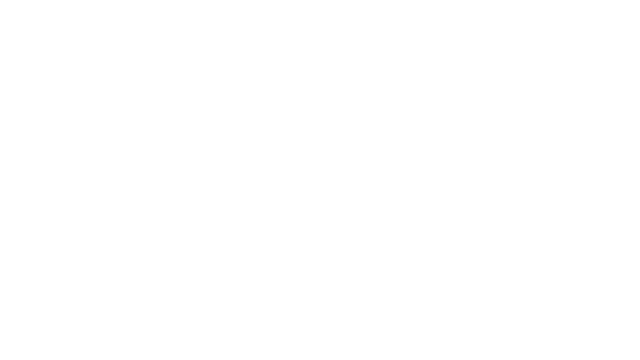 No magma. So we move on. Hope we have understood. Ha, The molten rock. The molten rocks are formed And why, when it comes to the surface, it is called lava. We continue. It is on to the earth's surface. 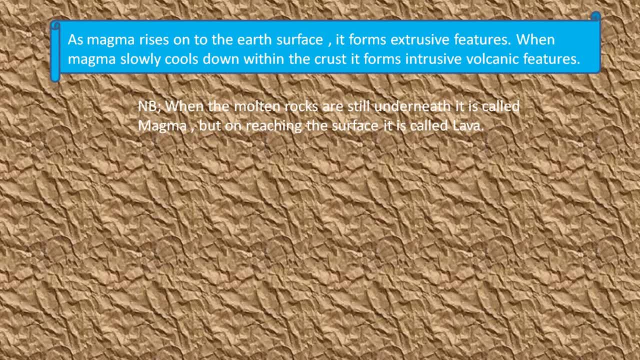 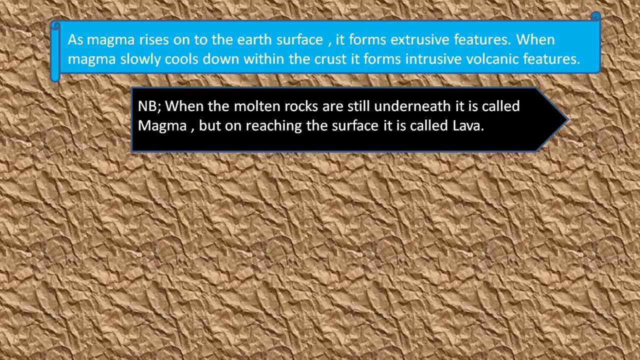 It forms extrusive features. when magma slowly cools down Within the crust, it forms intrusive volcanic features. Point to note here that when the molten rocks are still underneath it is called magma, But on reaching the surface it is called lava. 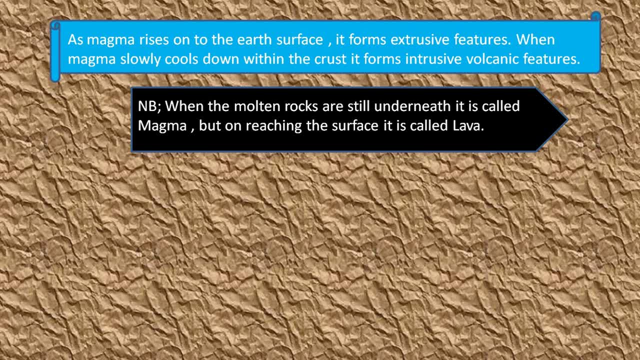 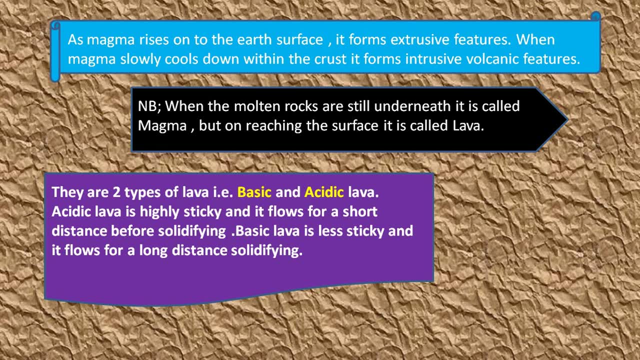 We have seen this earlier on. So we are saying: note this very well. So we are saying there are two types of lava, ie the basque and acidic lava. Acidic lava is highly sticky and flows for a short distance before solidifying. 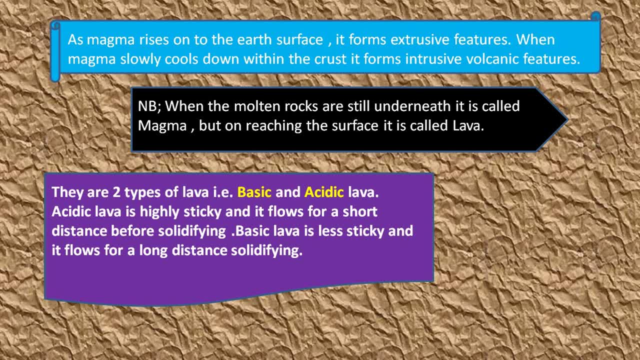 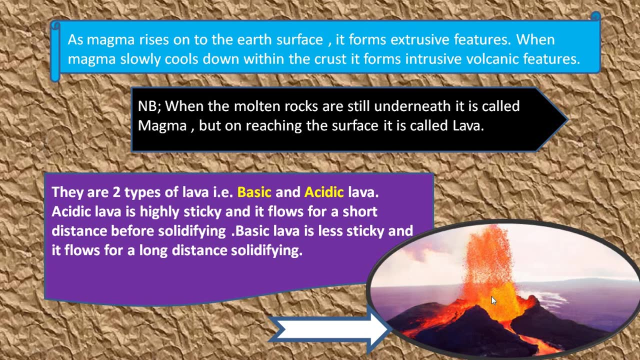 Whereas basque lava is less sticky and flows for a long distance before solidifying. So we are saying below here: we can just use this illustration to help us understand That what we see there in that photo is what we have just described as violent eruption. 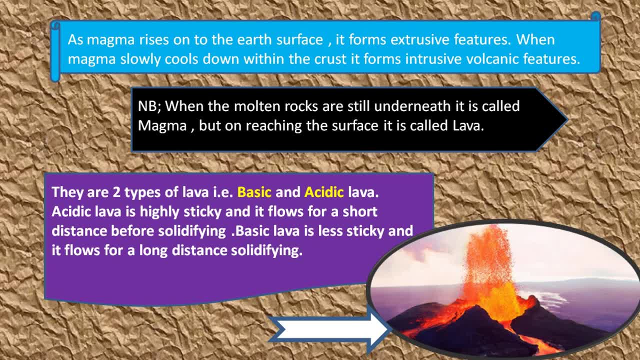 Where now magma has been able to be ejected onto the earth's surface. That's the crust, The surface of the crust, And we are saying, When this reaches the surface of the crust, we call it lava. So we are saying, when it is ejected violently, it will have to flow. 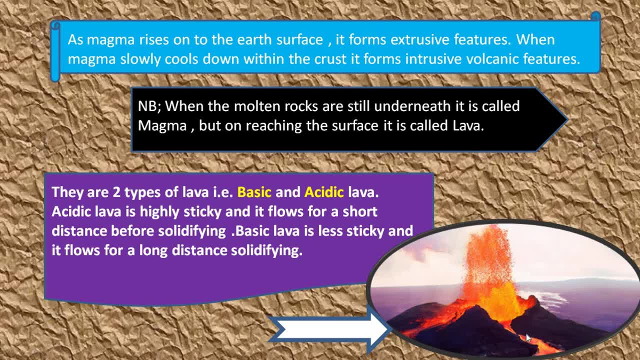 So this flowing that we see here, This one here, So when it flows for a long, long distance, that is called basque lava. But when it flows for a short distance from where it has been ejected And finally solidifies, it is called acidic lava. 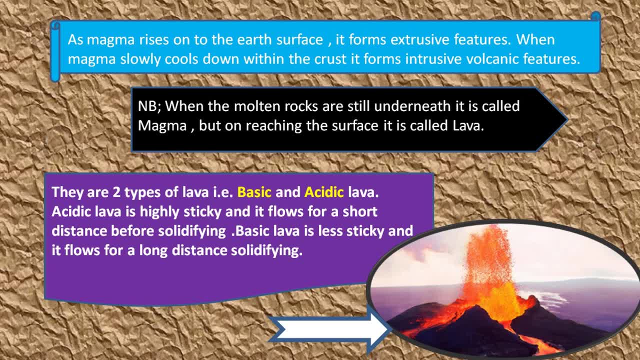 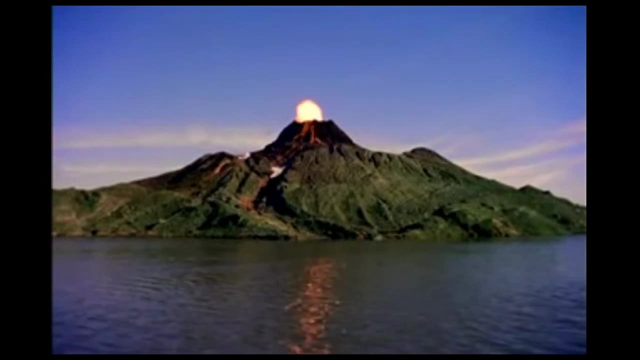 So below here, I want us to go into this video of volcanic eruption To help us understand what we have just talked about And, before we move on into the details of volcanicity as a topic, Enjoy the video. The next place in this video today: 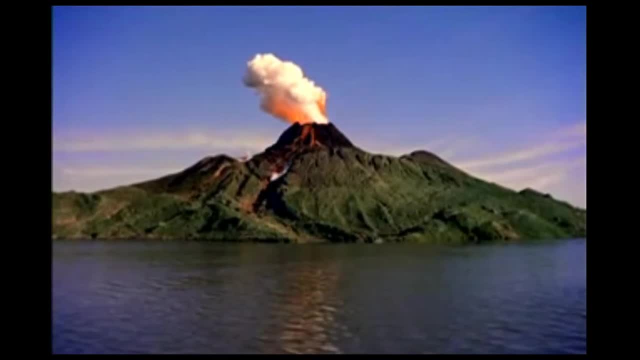 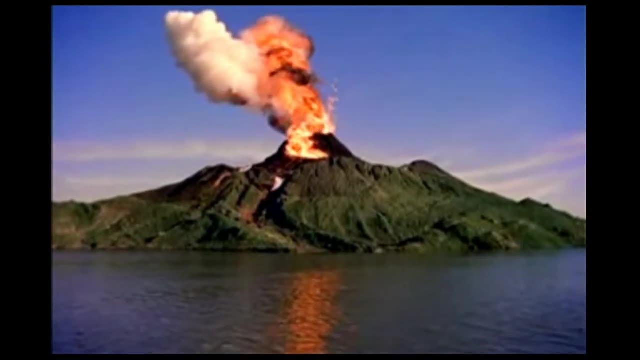 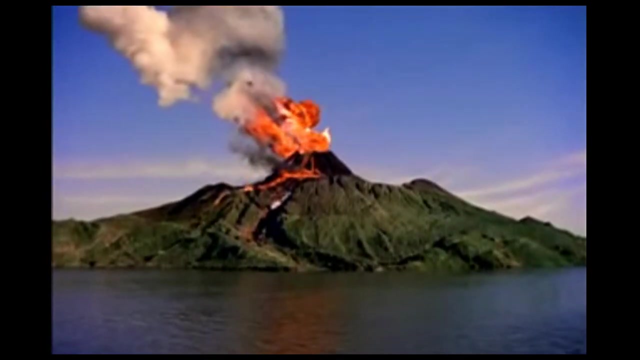 Oh, my goodness, Look at that. My goodness, That is smoke, fire and ash that comes out fast, That is fire, My goodness. Wow, Look at the intense pressure that happens. So it's due to the pressure that pushes the magma out onto the earth's crust. 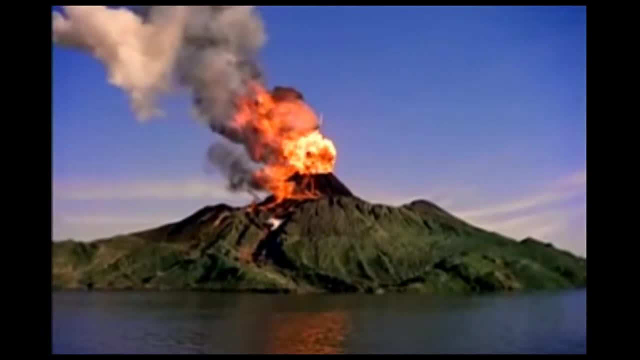 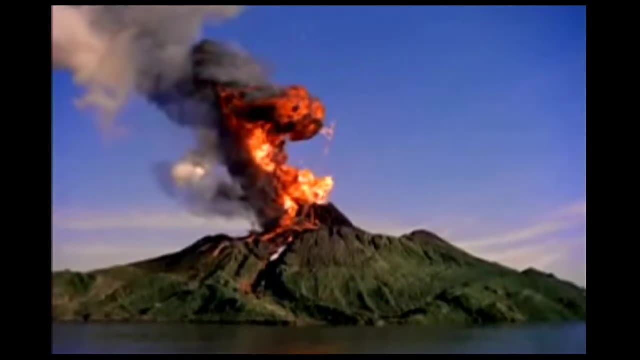 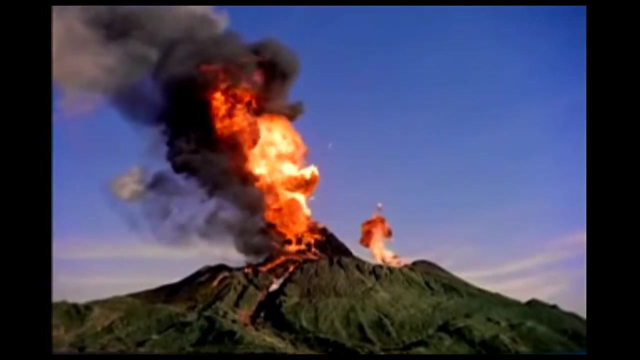 Which then turns into lava. My goodness, Look at that. Wow, So the top of the mountain has been blown off, And this is what we call the violent eruption. My goodness, Look at the eruption in the side vent. Have you seen that? 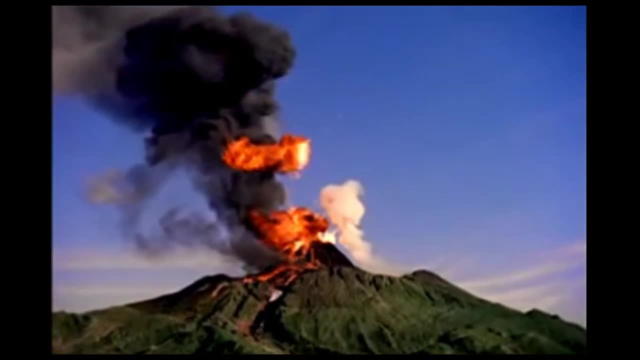 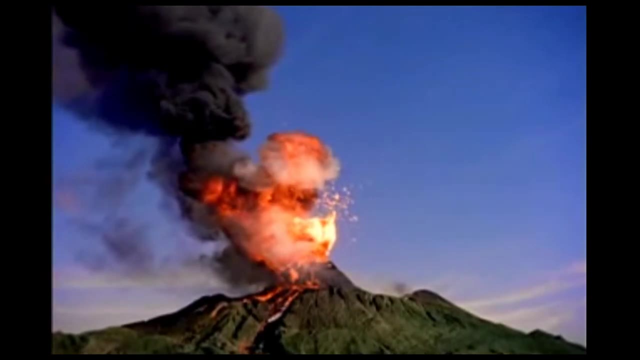 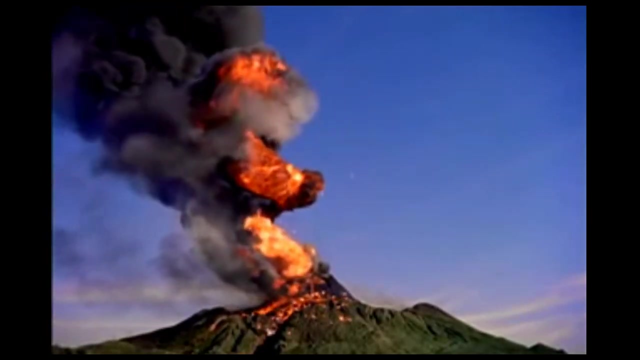 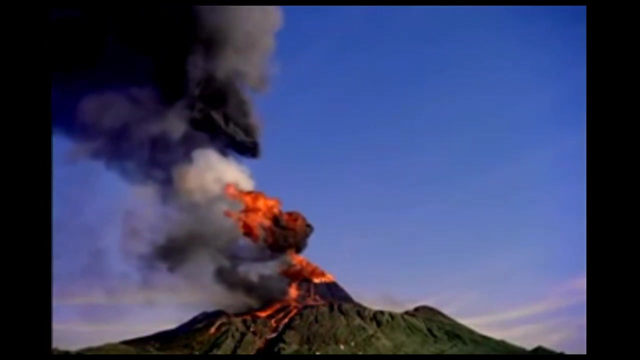 That's what we talk about in geography. This is, this is so, so amazing. So volcanic eruption is quite interesting. At the same time can be quite disastrous, As you can see. So it is throwing its magma fragments for quite a distance. 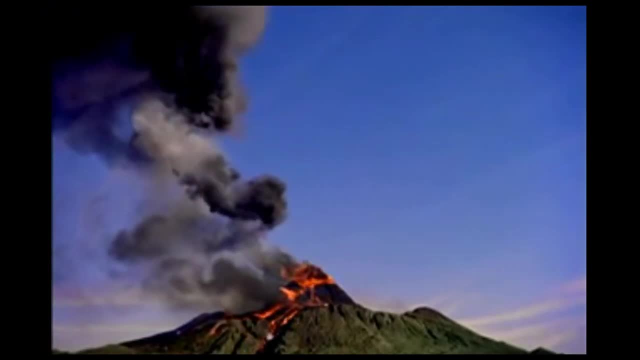 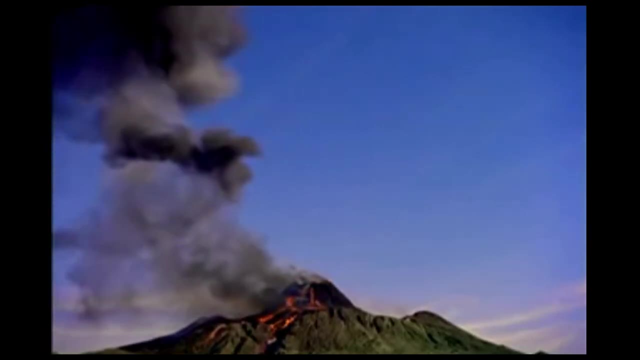 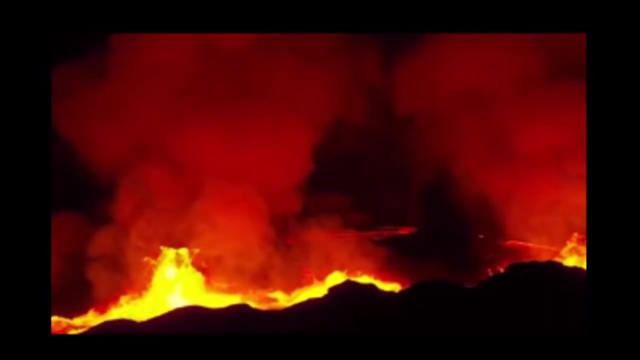 Hope you've seen that, My goodness. So this happens because of the pressure beneath, And we talked earlier. We say that the heat due to place the seat onto the crust forces the rocks into the mountain to be molten rocks, Which are called magma. 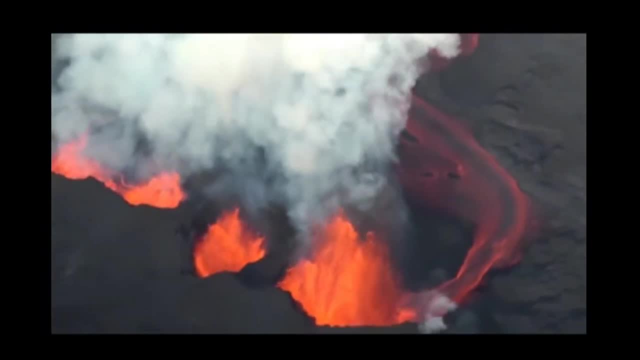 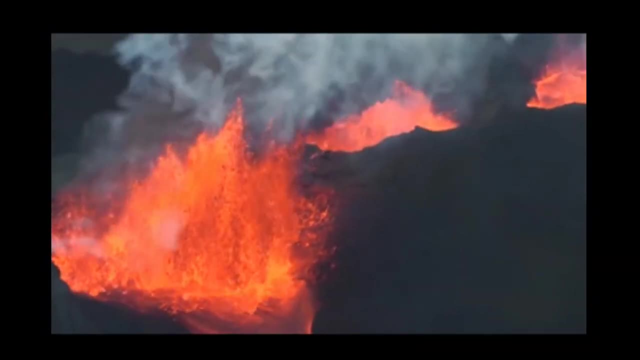 And the red stuff that we see here, The fire kind of stuff that we see here, Is actually the molten rocks. That's the magma we're talking about, But, as you see, the white is disappearing, The gas going out. Then, when it settles on the ground, 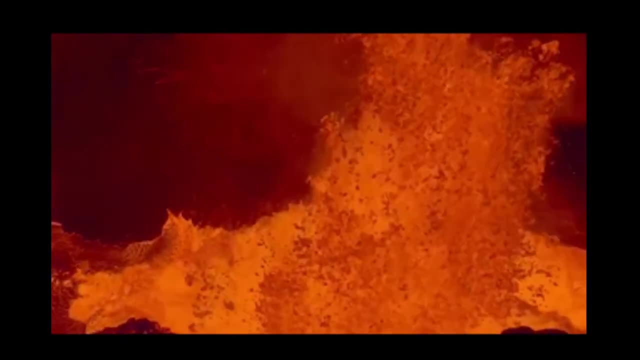 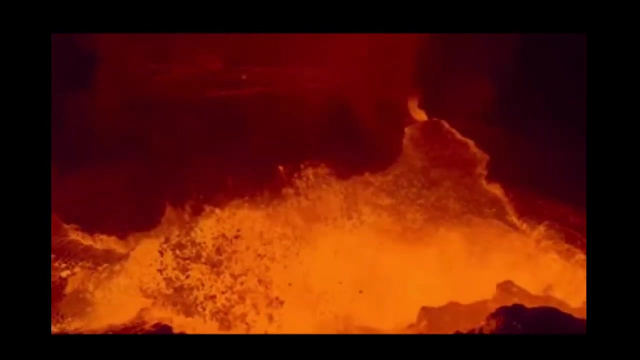 It turns into lava. My goodness, Look at that. That is fire. So when we say that igneous rocks are formed by fire, This is what we mean. This is what we mean. My goodness, God is great. Look at that. 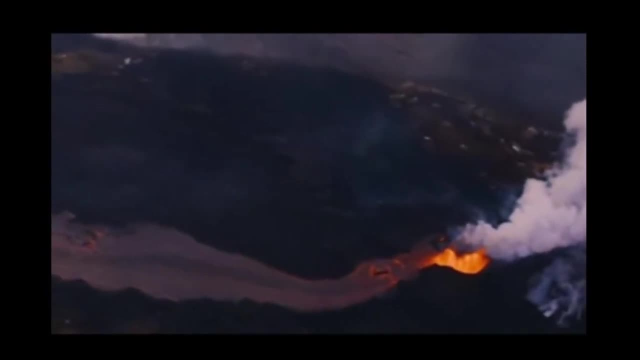 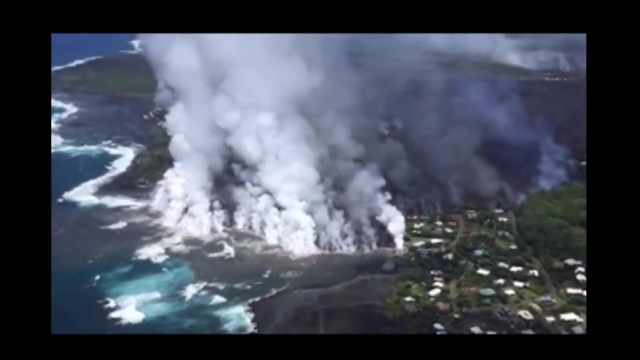 Just look at that. It's a boiling pot. So what we see down here is the floor We talked about being disastrous. You can see the houses burning. My goodness, Look at the lava floor. For quite distances It can be disastrous. 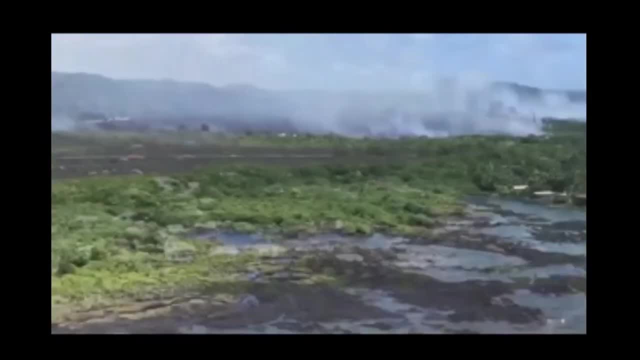 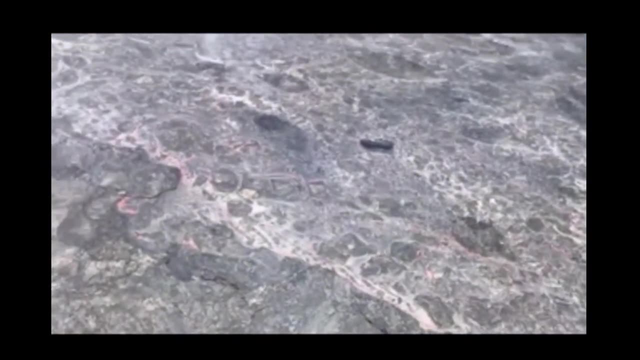 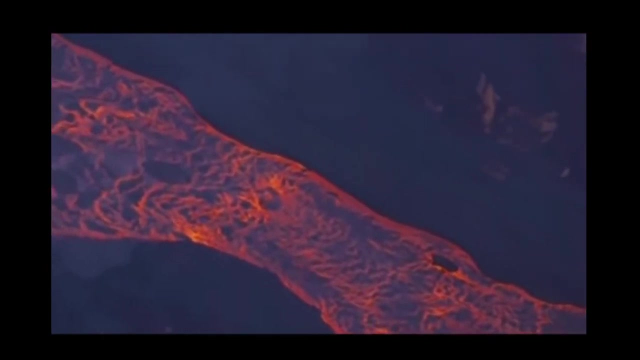 Thus destroying vegetation, animals and actually sediment. My goodness, What you see right now Is the lava floor. Actually, it has solidified. now It has blocked even the rod. My goodness, So we're saying Bask lava is the one that flows for quite a long distance? 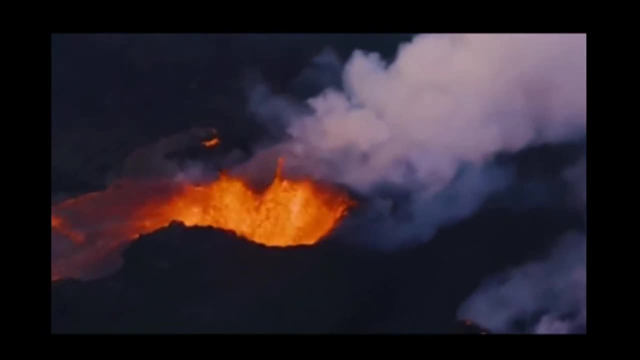 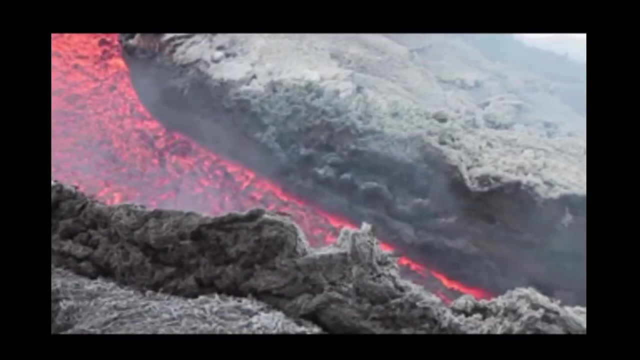 Then a civic for a short distance. So what you've just seen here that has flown for quite a long distance, That must have been besk lava. The one that you see right now in the video Is besk Going for quite a long distance. 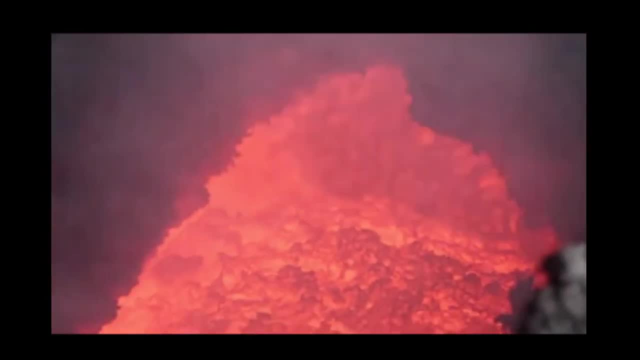 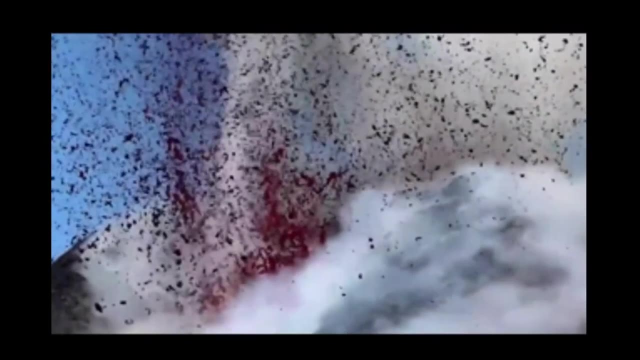 My goodness, That's fire flowing And that's the lava that we were talking about, So it will finally solidify and form the exclusive futures That we talked about. My goodness, Hope this video has helped you to understand what happens during volcanic eruption. 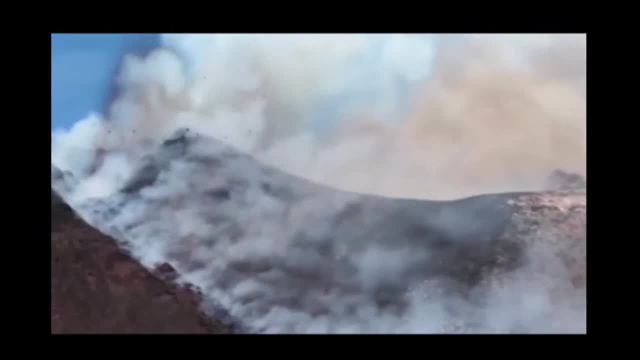 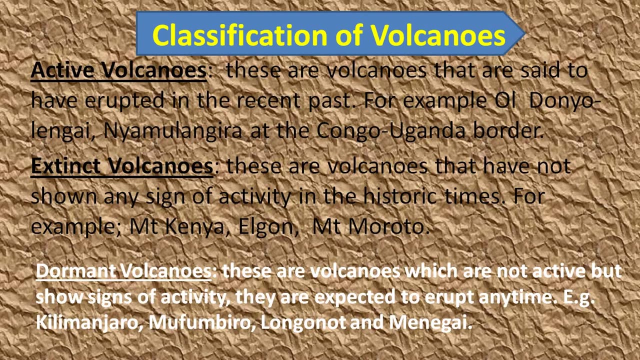 Thank you, I guess it was that lovely. So we want to look at the classification of volcanoes. What we have just seen there is the active ones. They're erupting And you've been able to see how the violent eruption happens. 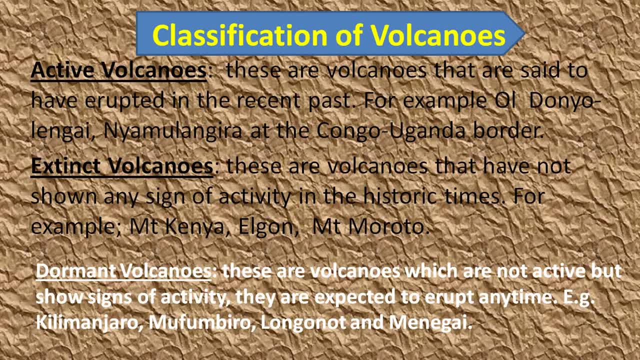 How the lava flows And how it finally solidifies. So I guess that video was just quite enough for us to understand what we are talking about And why we call volcanicity as one of the interesting topics in geography. So we move on. 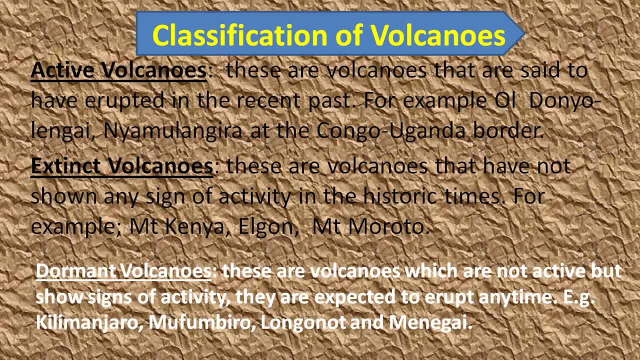 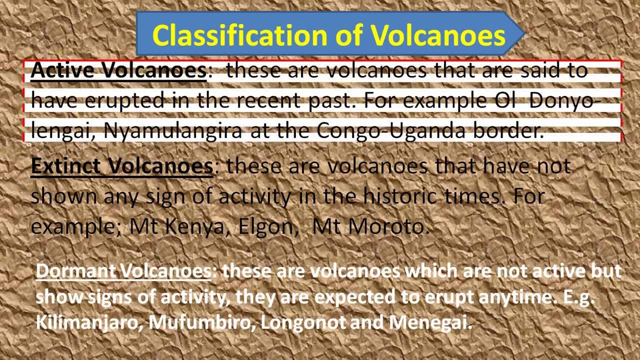 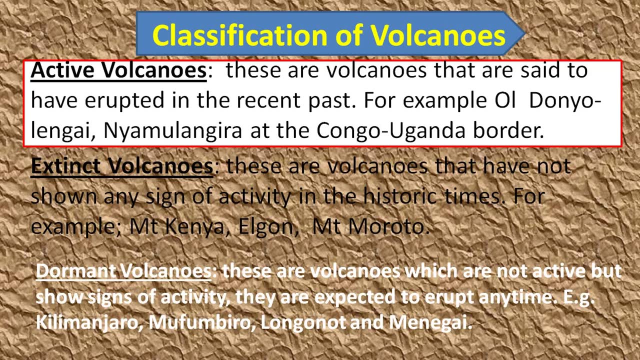 Classification of volcanoes. So we are saying: volcanoes are these futures formed by the process known as volcanicity? So we are saying Number one: We have what we call active volcanoes. These are the volcanoes that are said to have erupted in the recent past. 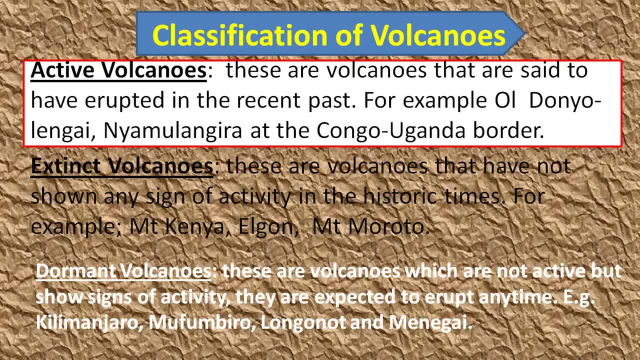 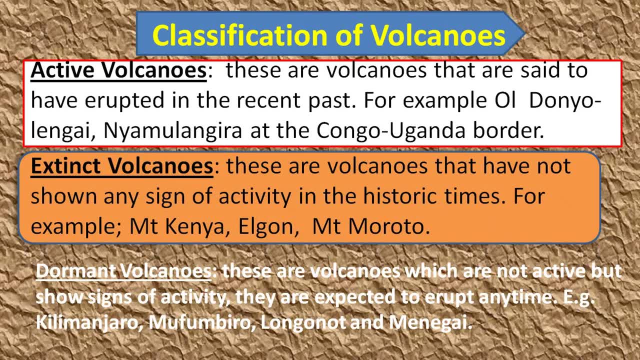 For example, In East Africa We have the Nyamlangira. At the Congo You get a bansin. We also have what we call the extinct volcanoes. These are volcanoes that have not shown any sign of activity in the historic times. 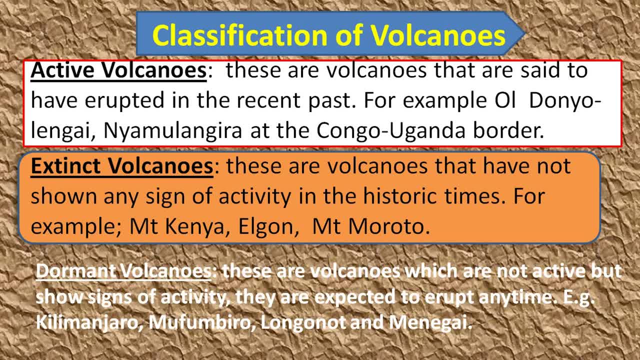 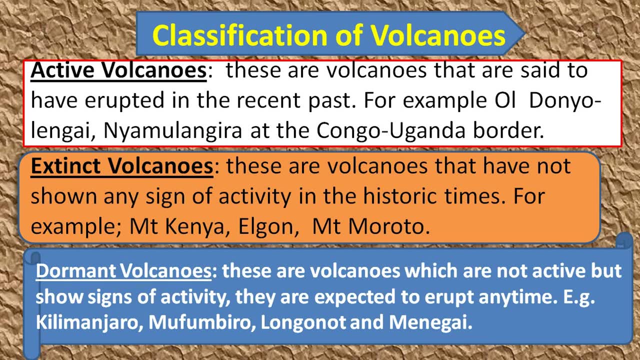 For example, Mount Kenya, Erigon And Moroto. They did erupt some time back, But in the few years past We have not seen any sign that shows that they are about to We continue. Then we have the last classification, known as dormant volcanoes. 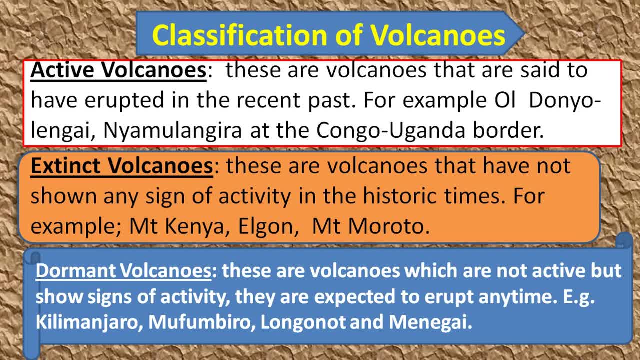 These are volcanoes which are not active, But showing signs of activity That are expected to erupt any time, Any time. You better be careful about it. For example, We have Chilimangiaramu Phumbido Long Knot. 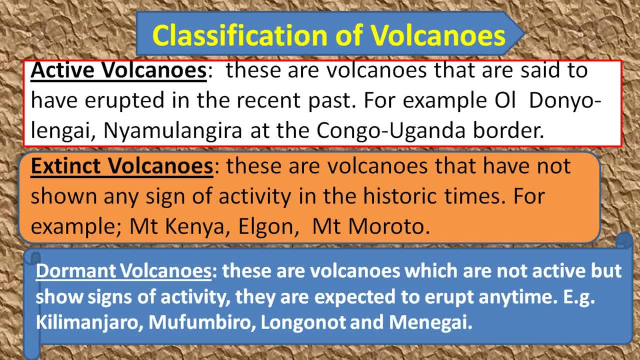 And Menengai, That is, in East Africa, Across the world Quite a number, Quite a number. But we are looking at the examples in East Africa So we are saying These ones are showing. These ones are showing some signs of activity. 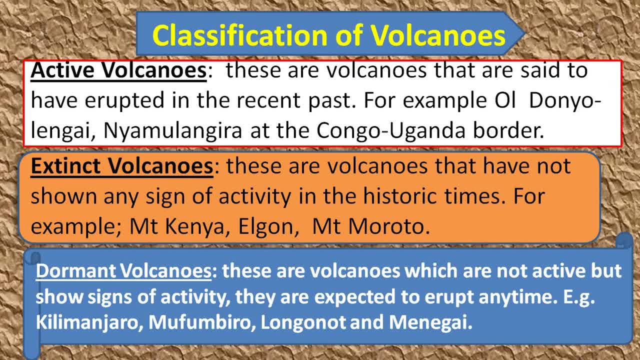 That are expected to erupt any time. So we are saying there have been dormant for some time. And these signs, For example, We can see the smoke, We can feel the temperature increasing, The animals living The steep areas of these islands. 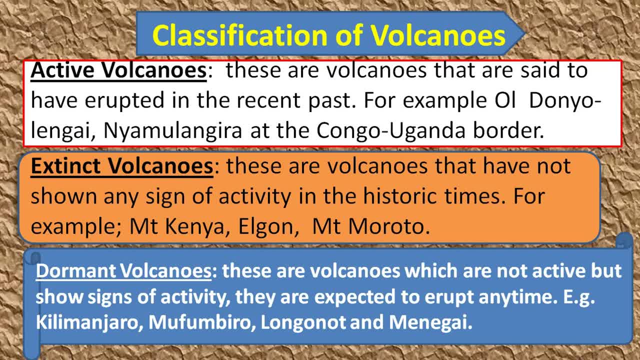 There are many, Quite a number of signs that show it is about. So we are saying The dormant volcanoes Are showing signs And have been so dormant for some time. So the classification that we have here are three Active volcanoes. 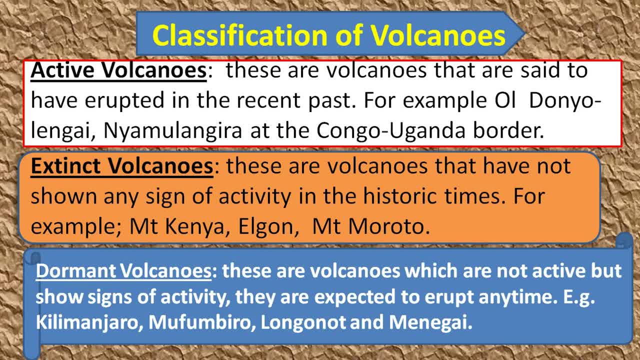 Extinct volcanoes And lastly, Dormant volcanoes. So we are saying Active. These are Volcanoes that are said to have erupted in the recent past. Some time back They did erupt. They are extinct Volcanoes. 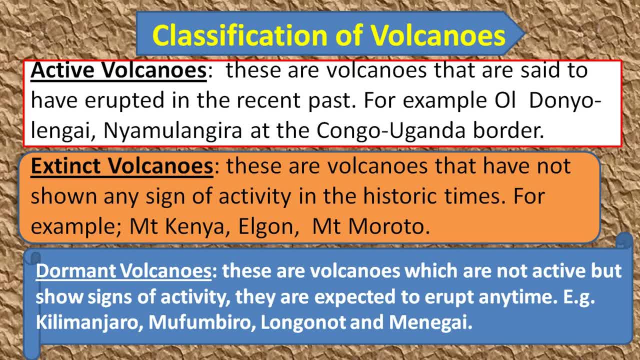 These are volcanoes that have not shown any sign Of activity in the historical times. So they have been there But they have not shown us any sign. Then, the dormant: They are saying: These are volcanoes which are not active But show. 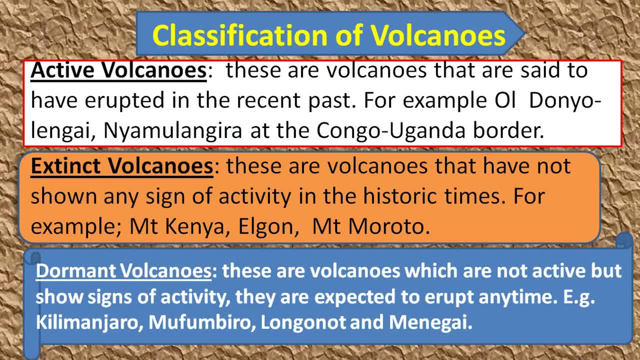 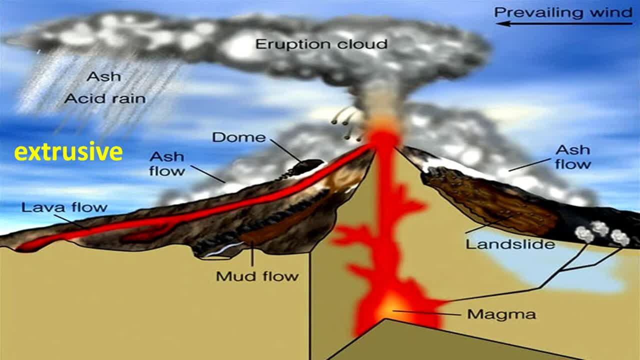 Signs of activity, We move on. So in this illustration We are Trying to bring out what we have just seen in the video Previously. So what we see here Is the process Of eruption: Magma coming out of the earth crust. 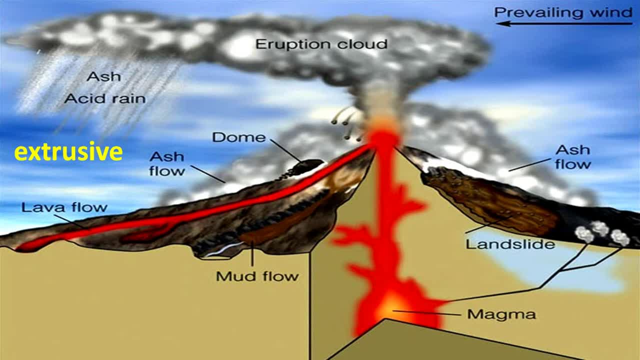 Onto The surface. So we are saying Extrusively is when It comes onto the surface of the earth. So what we see, That lava sloping down In that red colour. there Is what now we call The lava flow. 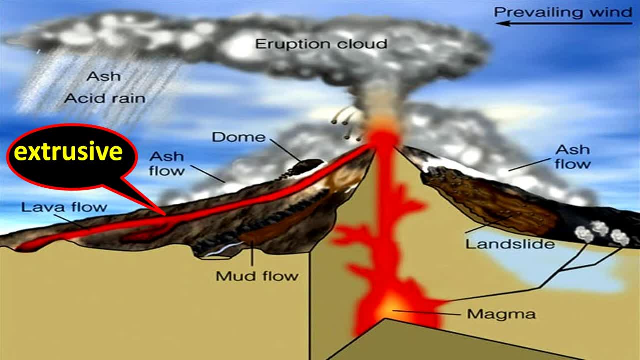 Which is flowing. We understood that we have the basic and acidic. One is sticky, The other is less sticky. So we are saying We can also have what we call intrusive, Where The magma has failed to reach the earth surface And it forms features like 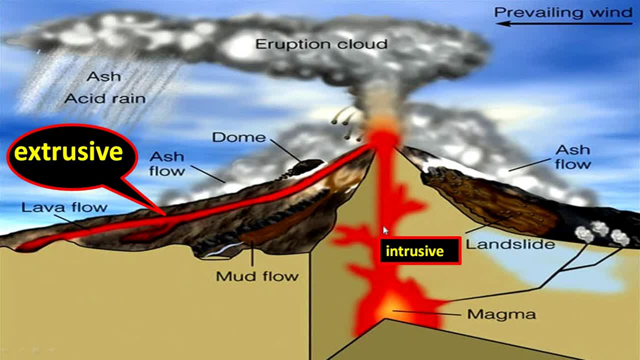 The sea, The dikes, The batholith, The larcholith And many others, As we shall see. So these are formed within the earth crust, But the other features, as we shall see, The dune, The composite cone, 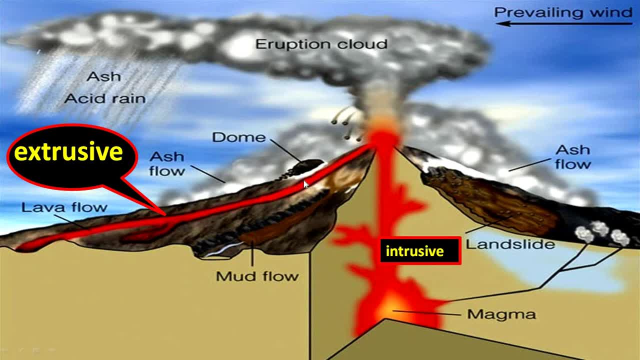 The crater And others Are formed outside The earth crust, And those are known as extrusive. So below, here is what we call The magma, And then it is Moving through the lines of weakness Which are caused by either faulting or falling. 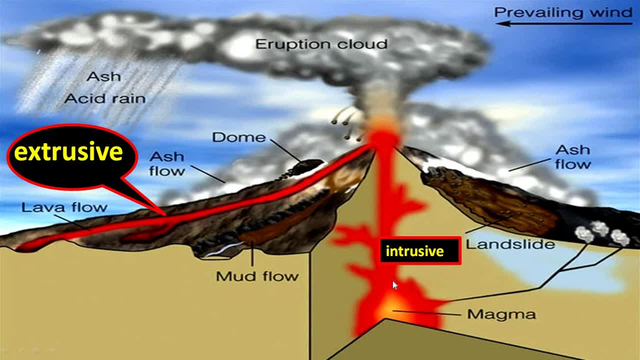 Onto the earth surface. And then we are saying What we see here is the eruption cloud. We say it starts with The dust And the gases, Then the ash, Before the magma comes. So this is the ash flow That we see. this other side. 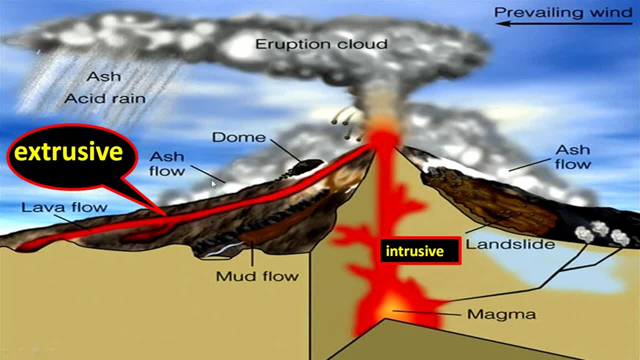 And this other side, Ash first, Then the muddy flow That was once in that area. So due to eruption, It is boom. Hope we are getting this, We move on. So we are saying We want to start with what we call. 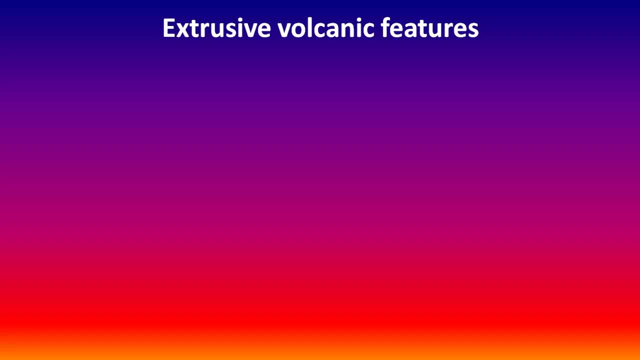 Extrusive volcano features, These, which are formed outside The earth crust. We are saying number one. We have the composite cone. It is made up of alternate, Successive layers Of lava and ash. It is formed through successive eruption And ash. 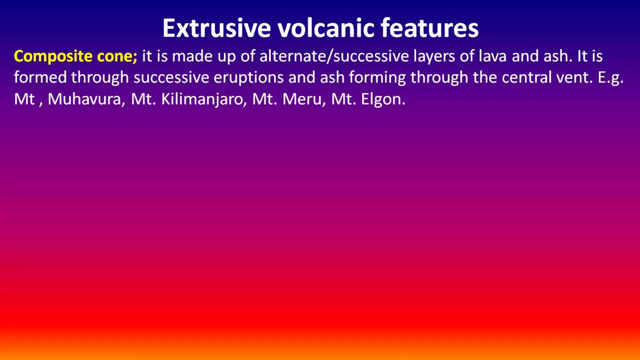 Forming through the central vent. So when Eruption takes place For quite some time Successively, The layers of magma Coming onto each other Are the ones that will form The composite cone, And examples of composite cone In East Africa. 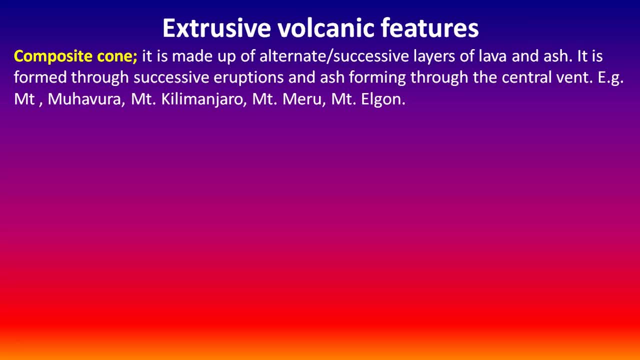 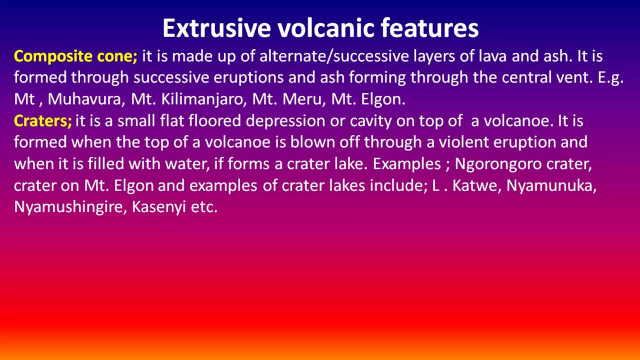 We have the Mount Muhabara, Mount Chilimanjaro And Mount Nehru, And then Mount Elegon. We move on Craters. It is also an example of Extrusive volcano features- Craters. It is a small flat. 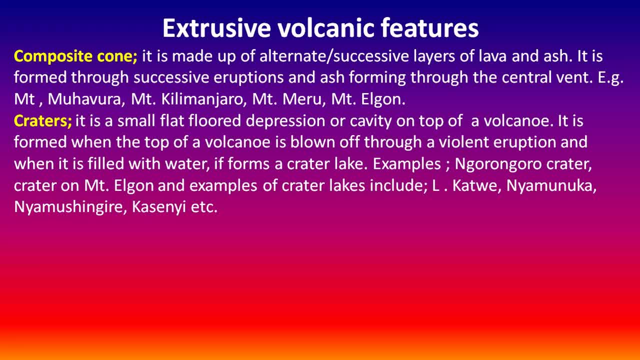 Flood depression Or cavity. The volcano is blown off Through a violent eruption And when it is filled with water It forms crater lakes. Quite a number. in East Africa We have quite a number, For example The Queen Elizabeth, Kind of a gem power. 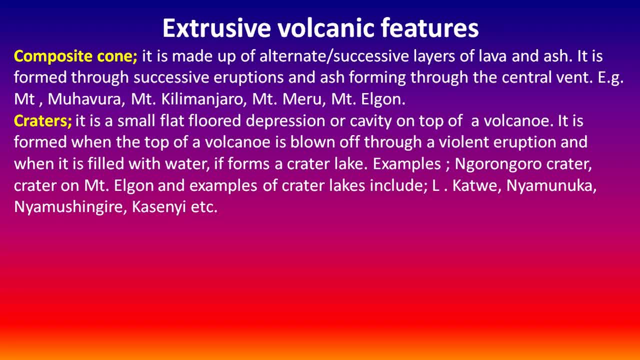 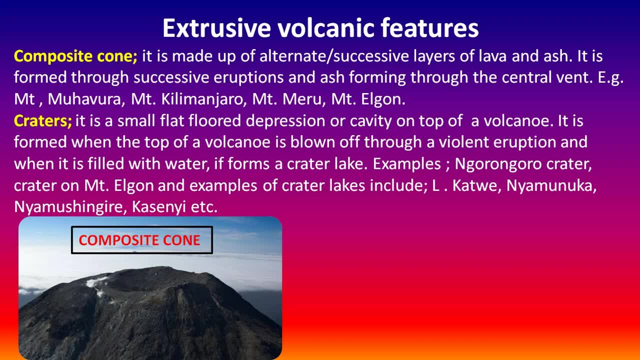 Quite a number, Quite a number, And the examples are given below. here We move on. So we are saying: This is A diagram, A photo to show us How a composite cone looks like. We are saying It is made up of alternate stroke. 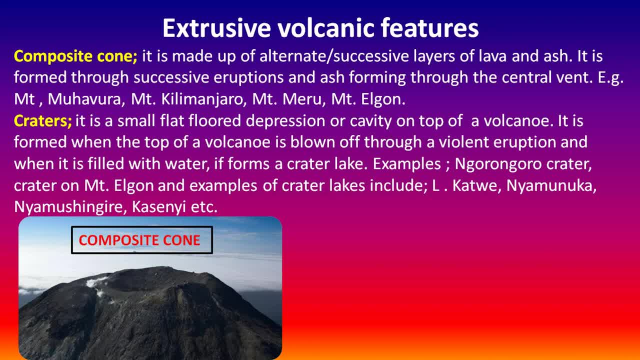 Successive layers of lava. Lava, Remember we said, lava Is the one that comes on the earth surface Where the gases disappear. It is not magma now, It is lava. So successive layers, As we can see This one here. 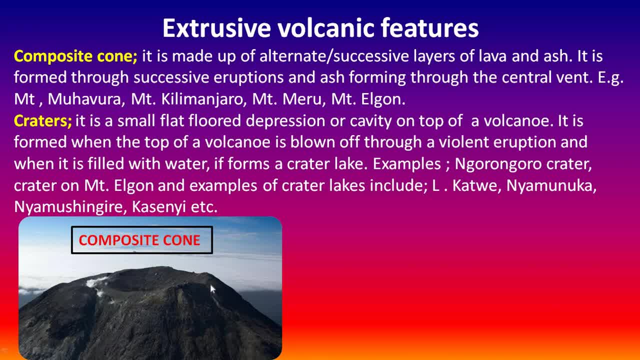 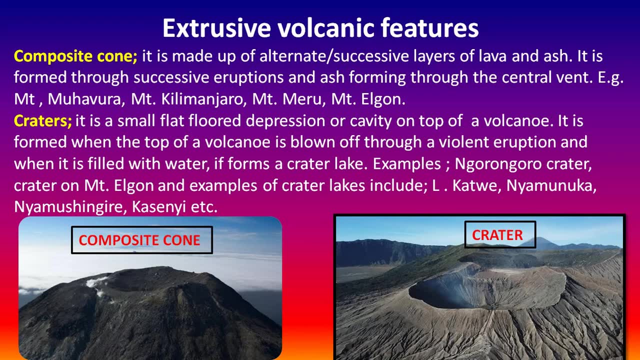 The layers of lava Flowing Due to continuous Kind of eruption. It forms a composite cone. We move on This other side. We are seeing what we call A crater And we are saying It is a small, flat flowed depression. 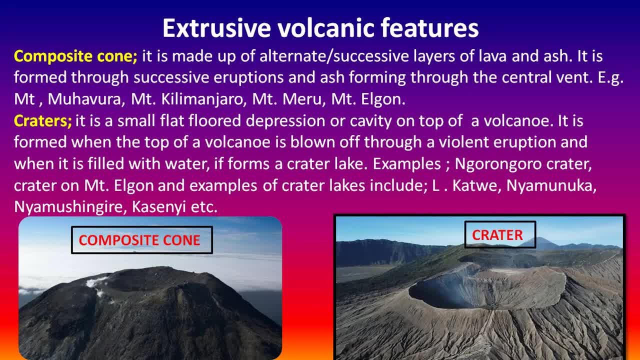 Or cavity On top of a volcano, It is Blown. when the top of a volcano Is blown off Through violent eruption, This is what we are seeing down here, That what you see here Is a small, Not actually small. 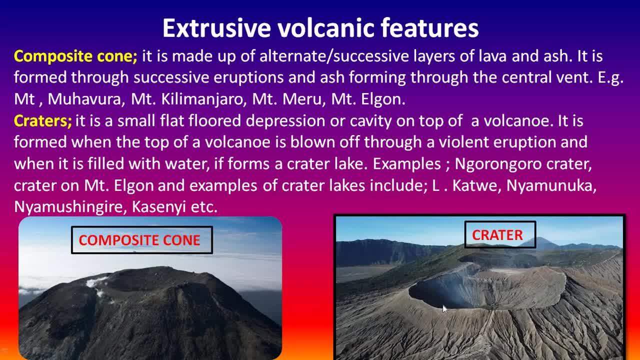 It is big, But a sharp kind of depression. Cavity On top of this volcano Is blown off When violent eruption happens. So this Can help us understand What we always look at Theoretically. Now practically, We can see this in photos. 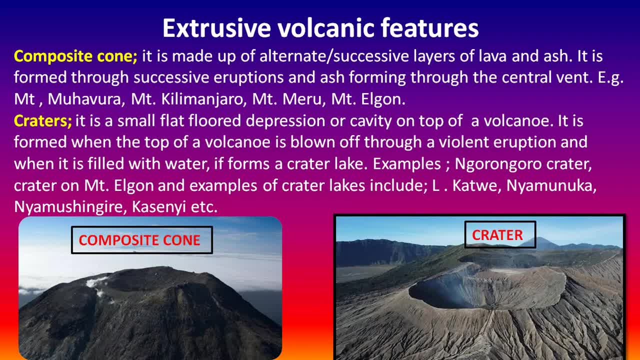 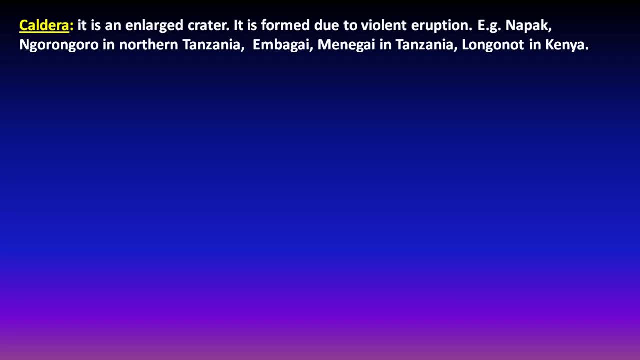 And understand them better. We move on. Other features of Extrusive volcanic features. We move on. We have the caldera. It is an enlarged crater. Remember we have seen The crater initially, But now this is a caldera. 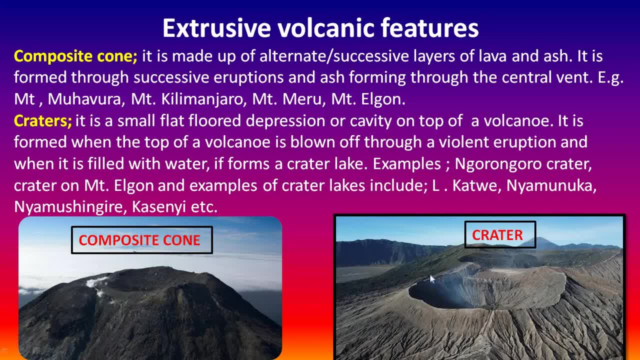 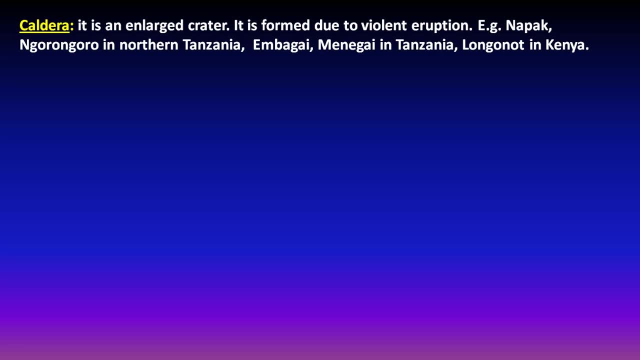 I can take you back to a crater. This is the crater We were talking about, But now it is enlarged Due to the erosion process. It is going to be called A caldera, So we think It is an enlarged crater. 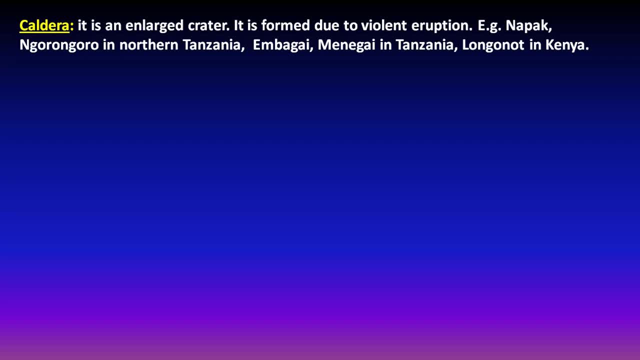 It is formed due to violent eruption. Examples in East Africa: We have the Napaque Ngorongoro. in Northern Tanzania, Mbangai Mnangai. These are examples in East Africa. Across the world There are quite a number. 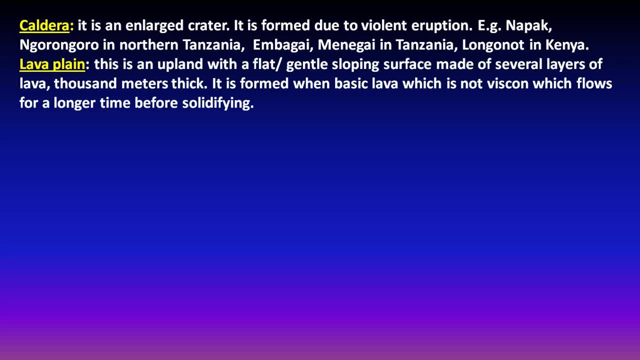 Many. Next is lava plains. This is an upland With a flat, Stroke, gentle, sloping surface Made of several layers Of lava Thousand meters thick. So we say it is formed When basic lava, Which is not viscous. 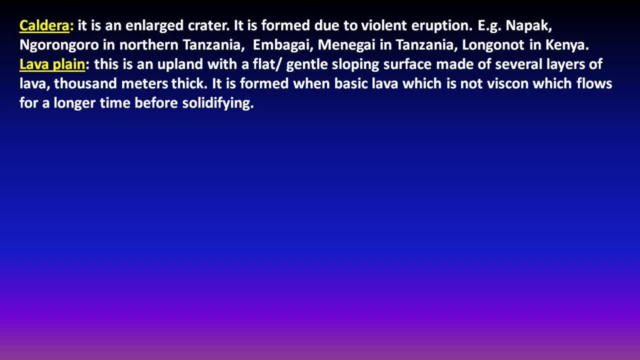 Which flows, Oh, not sticky, Which flows for a long time Before solidifying. So this lava is able to flow Quite kilometers, Quite meters Without solidifying. So when it flows For quite a long distance, It forms what we call. 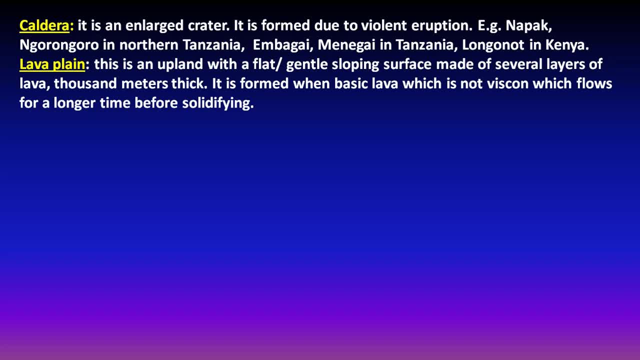 The lava plain. The lava plain- Hope we are together. Next we have Volcanic Plague. This is formed When molten lava Solidifies in a vent And later exposed On the earth's surface By processes of erosion. 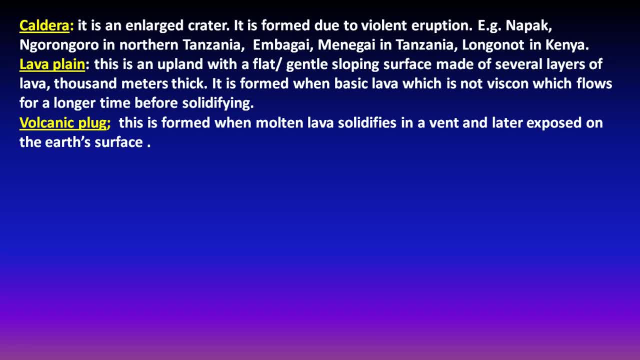 Denudation kind of processes. So it is Within But later exposed. Then ash and cedar cone. These are small, Symmetrical cones. They are cast Less than 150 meters With fairly steep sides Between. So we are saying: 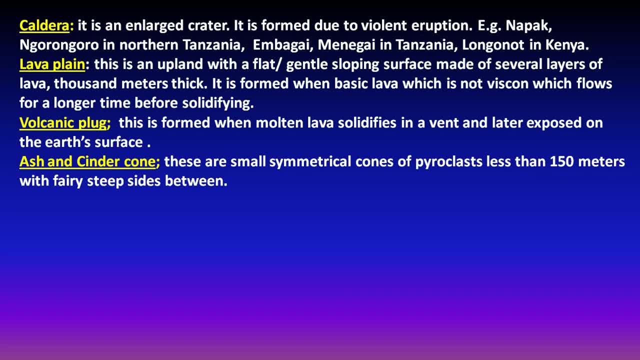 Ash and cedar cones. They are small, Symmetrical cones On top of these volcanoes Where the vents, Where the outlets of the volcanoes Were, So they form As, Due to the successive Eruption, Wind finery stops. 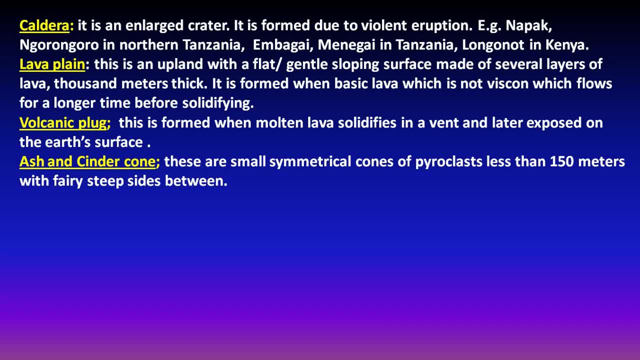 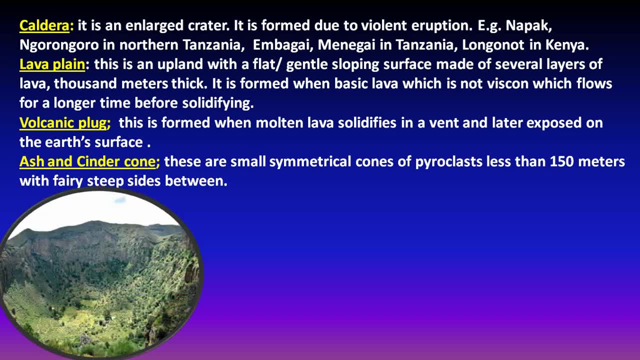 The lava that solidifies Around that area Forms a cold. So below here We are saying This is a caldela Wide. So we are saying it is An enlarged kind of crater Due to erosion. So it is wide. 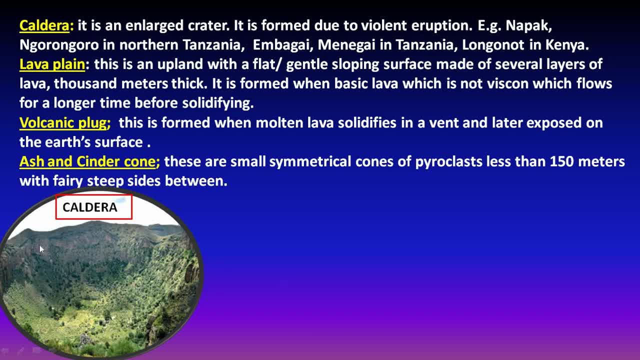 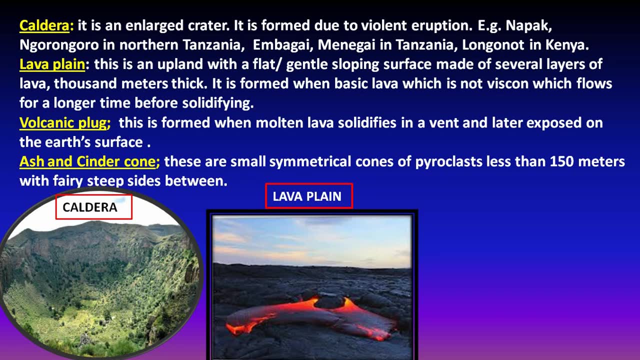 What we refer to as A caldela Quite, a number also In areas of Fort Potro. Then next is The lava Plain. This is lava Which has been flowing quite for A long, long, long distance And we are saying: 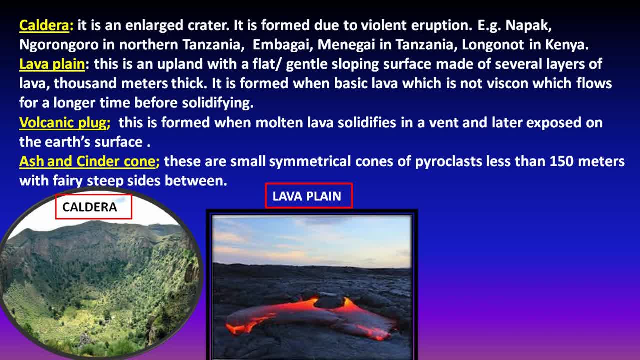 This type of lava Is known as Plain. So Here what we see here: This one is not yet even, Has not yet even cooled down. You can see, it is still Red. This other black one has already cooled down. 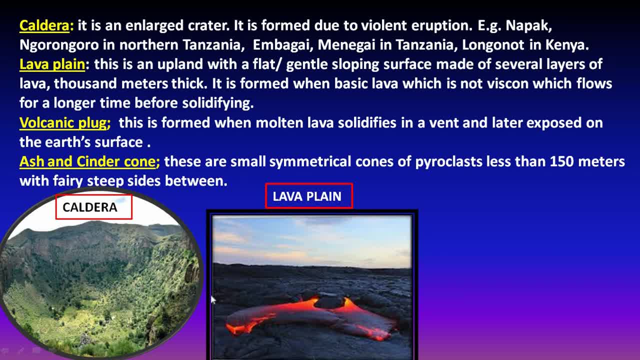 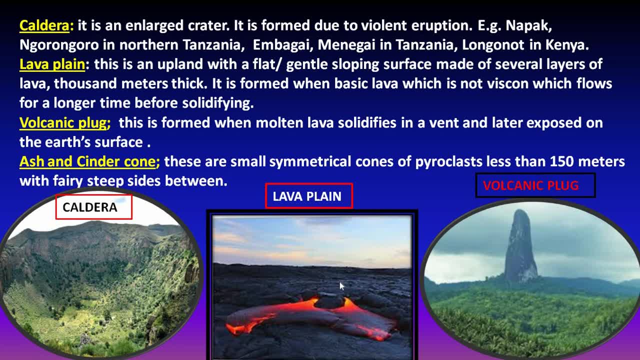 So this Expanse, kind of Extensive kind of area Of lava Is what we call The lava Plain, The volcanic Plague. Examples of this: in Uganda We have the toro rock. So it comes out of. 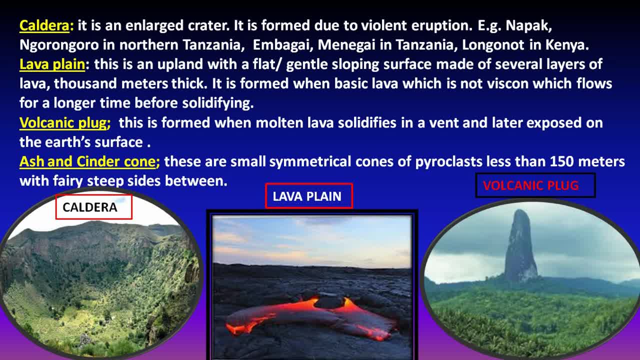 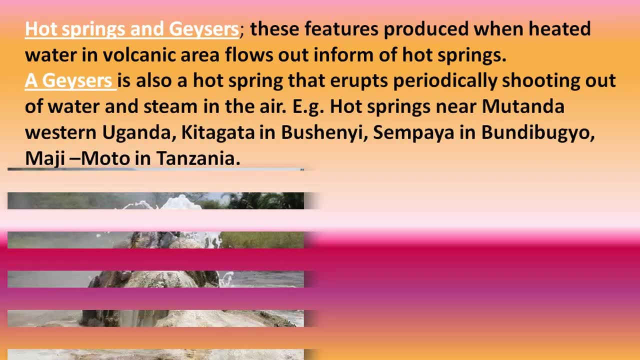 The ground. This was lava Trying to come Into the earth surface, But it solidified within The vent, And that what led to the formation of A volcanic plague. Now we have others: The hot spring. These are features produced. 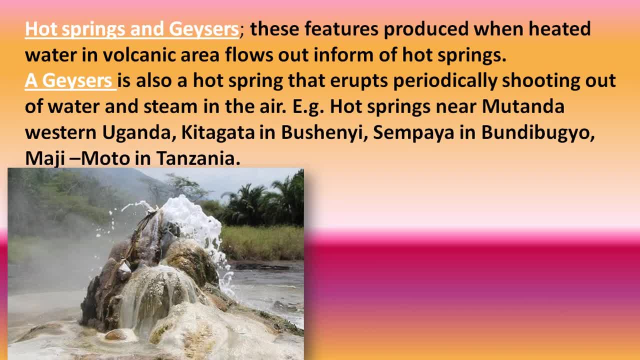 When heated water in the volcanic area Flows out In form of hot spring, Then the gisaz is also a hot spring That erupts periodically, Shooting out of water And steaming the area. For example, hot springs Near Mtanda. 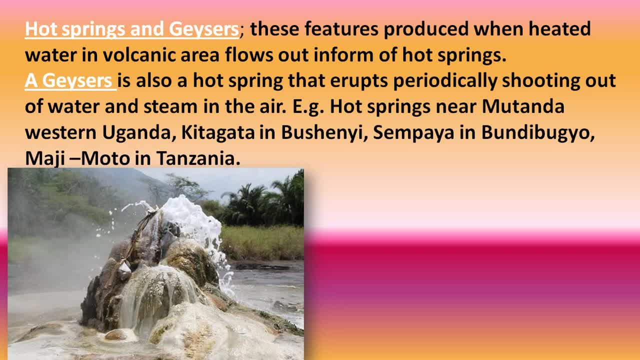 Chittagata, Sempaya, Majimoto In Tanzania, Quite a number The volcanic kind of Areas. We shall understand the geography Of the water spring, But now we are looking at Future's form Which takes to see. 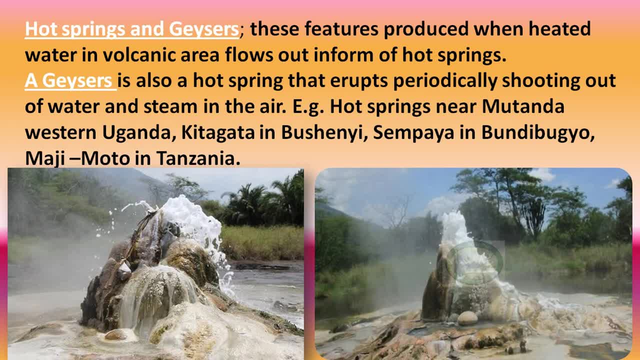 The kind of volcanic. So these are examples of Pictures trying to show us The water springs. Later in this lesson We shall have a video about them So you can see This is water, Really hot water. You can see with the steam. 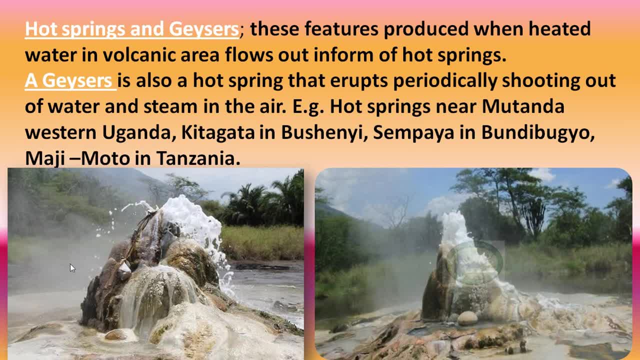 Here And it is due to the hot Temperatures Within The earth crust. As we said last time when we looked at the lava Or the magma is hot, So the temperatures Caused by this Different layers exerted 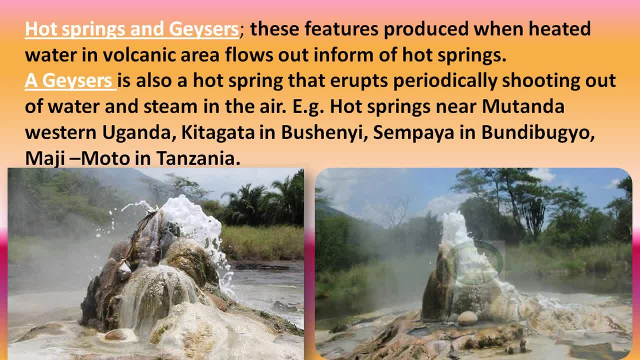 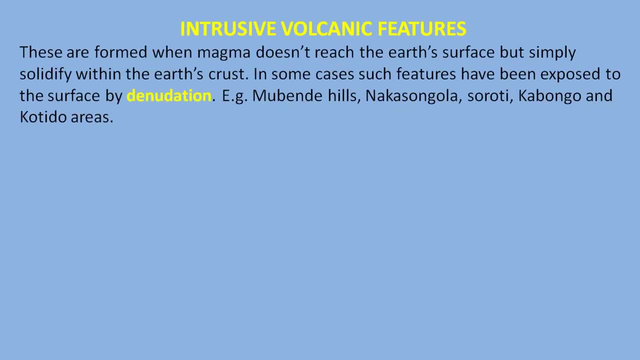 Onto the crust. They increase the temperatures, Actually Have boiled this water As it comes onto the surface, Forming the hot spring. We move on Now. we move on to the Intrusive volcanic futures We have been looking at. 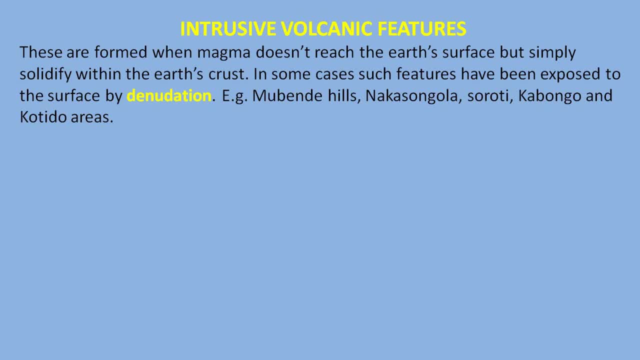 Extrusive things outside. Now I want to look at things inside: Intrusive volcanic futures, And this will conclude our lesson today. These are formed when magma Does not reach the earth's surface, But simply solidifies Within the earth's crust. 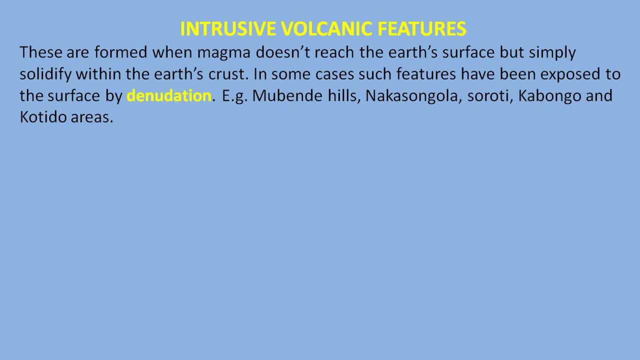 In some cases, Such futures have been exposed To the surface, by Denodation, For example. We have quite a number- And these are examples within East Africa Across the water, Quite a number. So these include The lapolith. 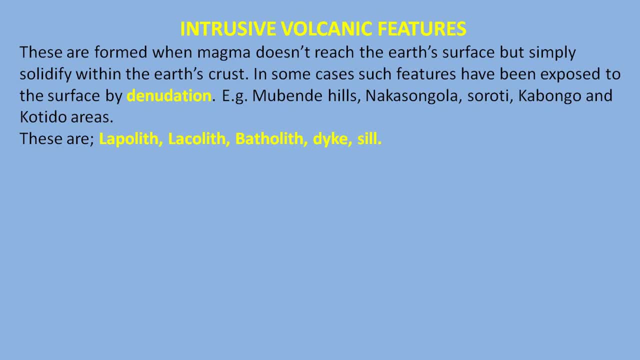 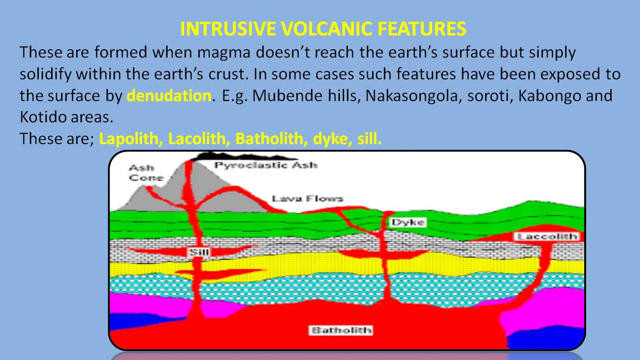 The narkolith, The batholith Lava does not go out Or outside the crust, It just slowly solidifies Within the earth's crust, Forming such futures. So below, here Is the photo To just briefly show us. 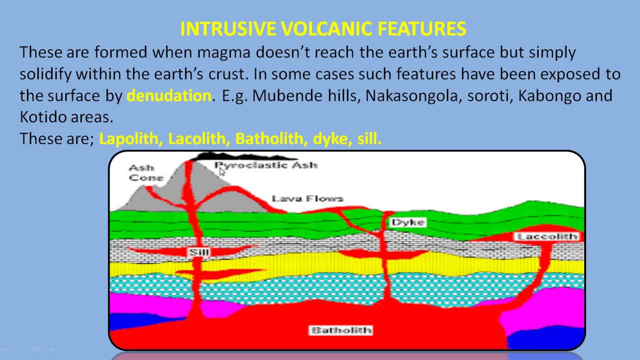 So this is outside, Outside. We talked about the ash corn, Remember In extrusive, But now we are interested In Those ones That are formed within the earth's crust, Not outside the earth's crust. So we have the dyke. 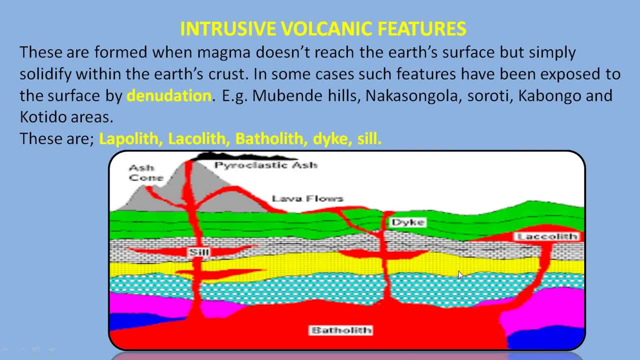 We have the batholith, We have the seal And then we have The narkolith. So these are futures Formed within, Within The earth's crust. Magma solidifies Within, Does not reach the earth's surface. 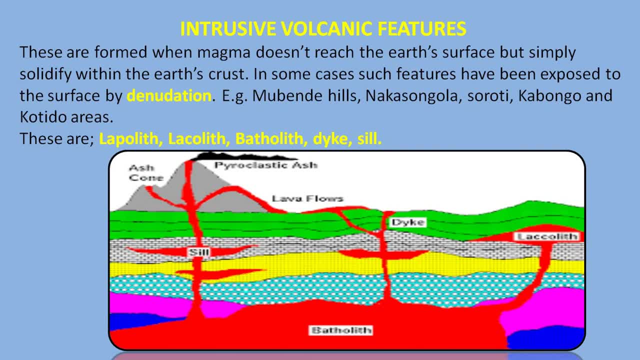 So with this We will have to end today's lesson, And I will leave you with A video of the hot springs That will help you to understand What you have just been looking at. Thank you very much. See you next time. 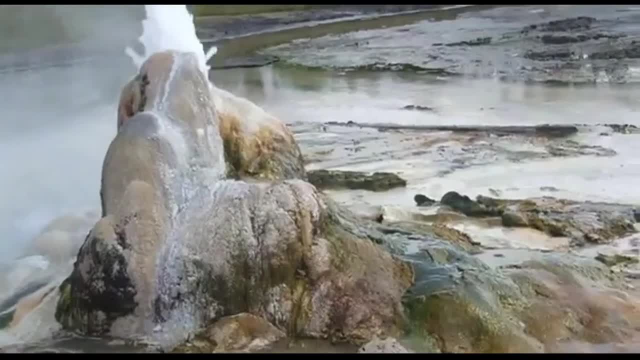 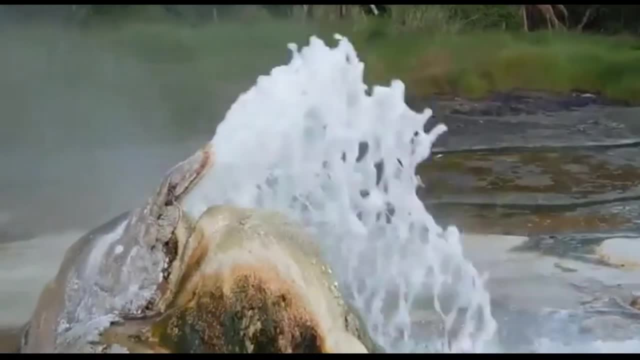 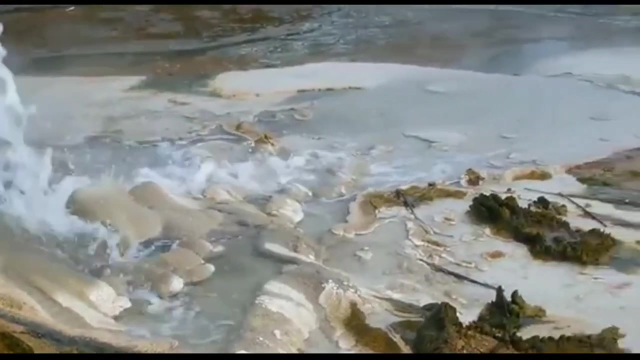 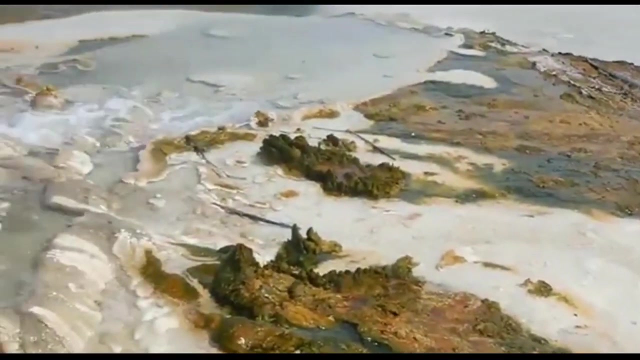 Bye, bye, Thank you.